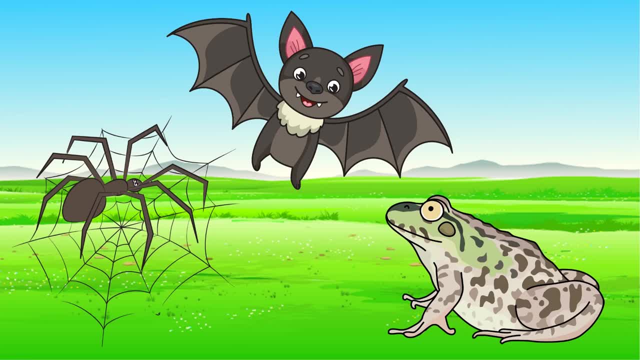 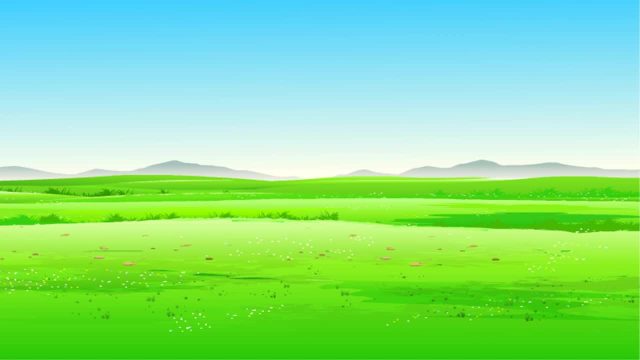 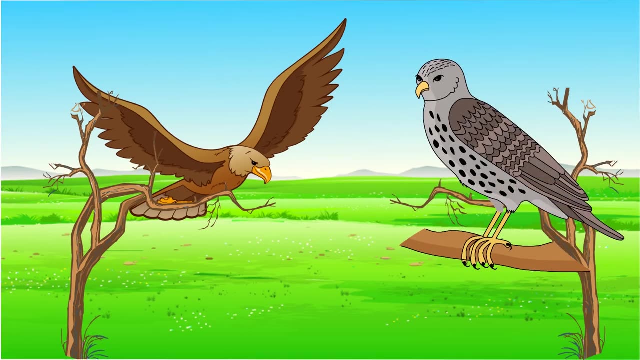 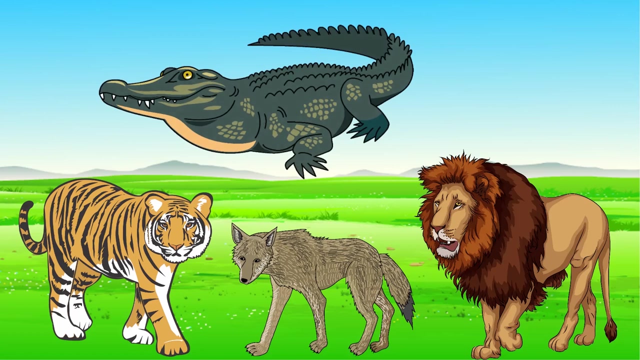 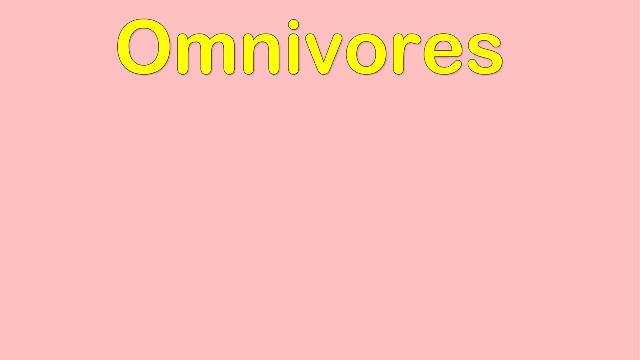 Spider, Frog and Bat are small Carnivorous. Medium size Carnivorous are large birds such as eagle and hawk. Lions, tiger, wolf and crocodiles are large carnivorous, Omnivorous- Any animal that can eat both plants and animals. 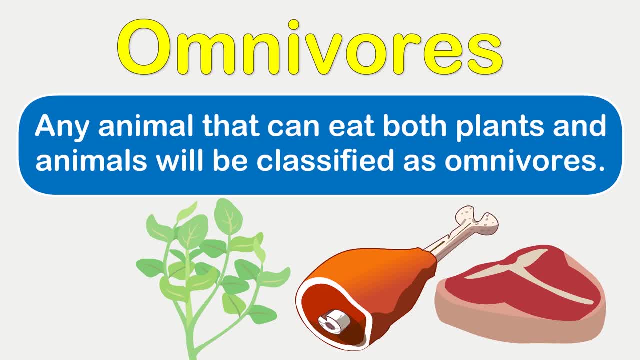 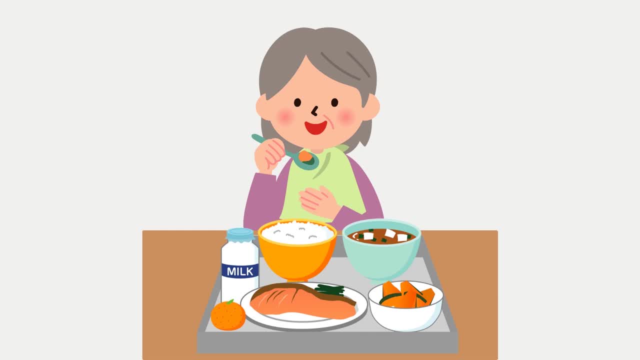 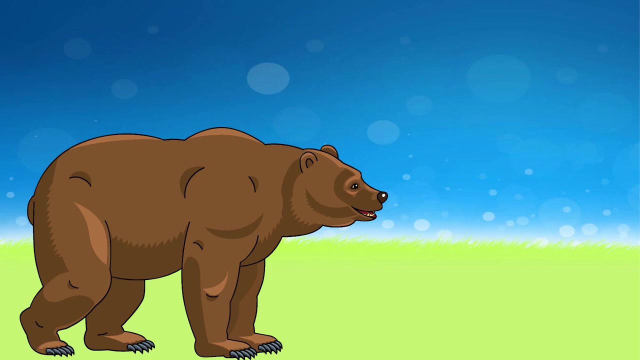 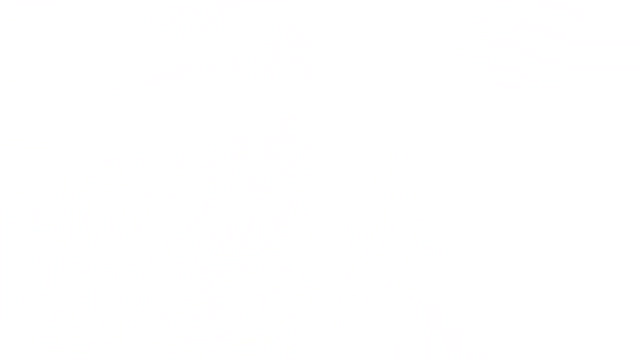 will be classified as omnivorous. Omnivores are omnivorous, containing flat and sharp teeth and the ability to digest meat, fruit and vegetables. Weirs are another example of omnivorous, as they eat both plant and meat. Chickens are another example of omnivorous, because they eat seeds and vegetables. 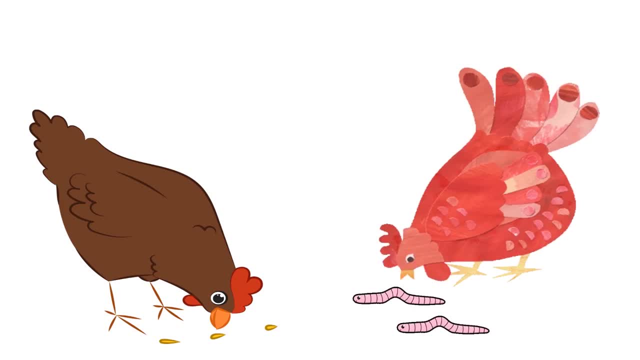 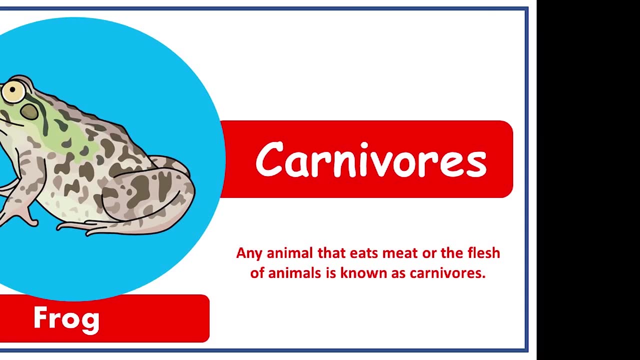 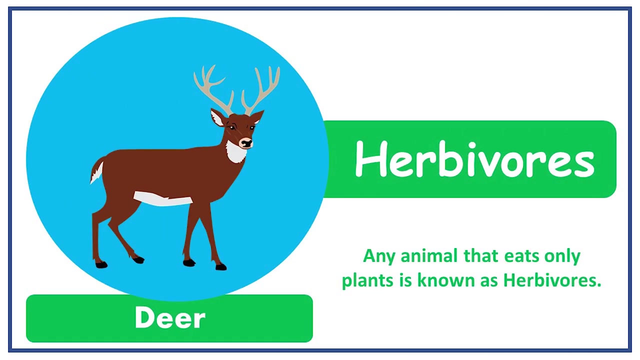 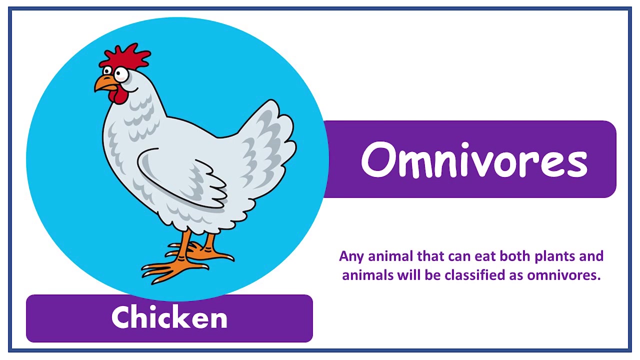 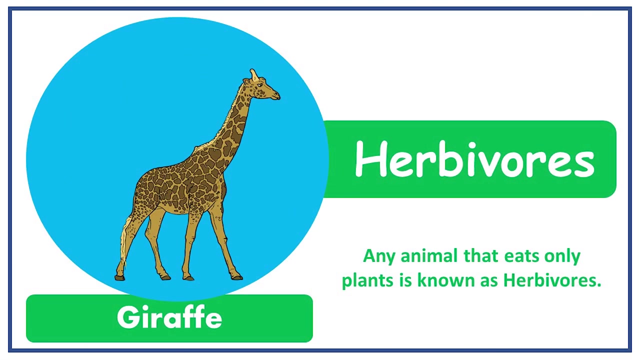 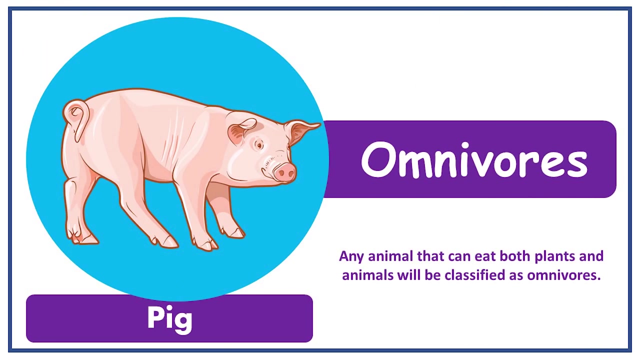 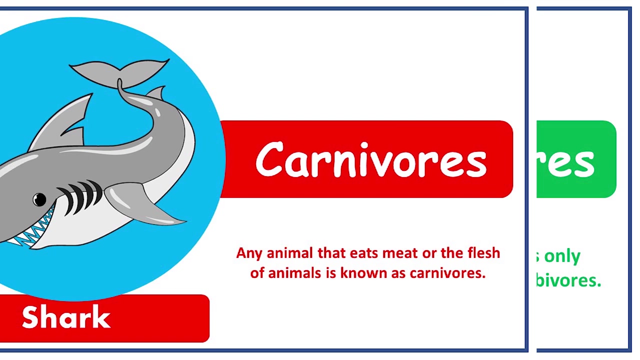 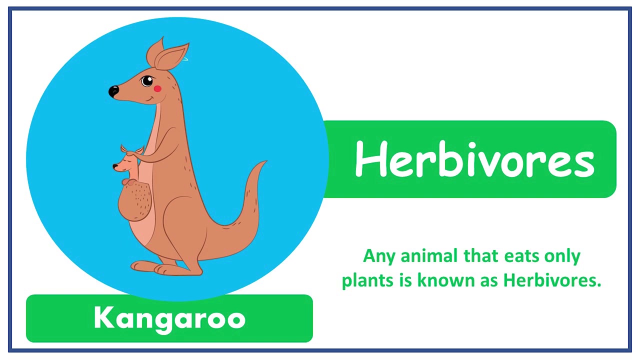 But they can also eat worms. Frog is carnivorous. Deer is herbivorous. Chicken is omnivorous. Wolf is carnivorous. Giraffe is herbivorous. Pig is omnivorous. Goat is herbivorous. Shark is carnivorous. Kangaroo is herbivorous. Buffalo is herbivorous. 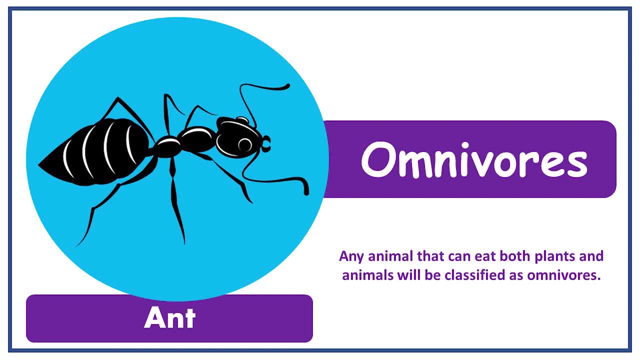 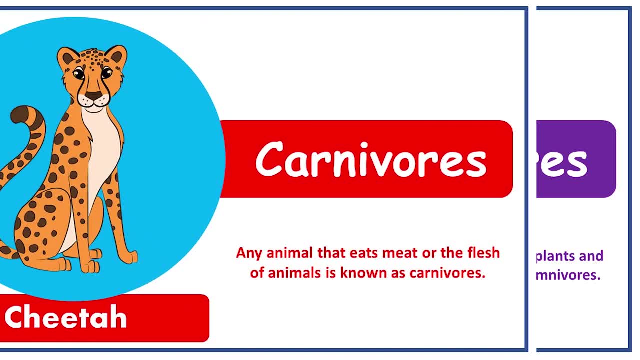 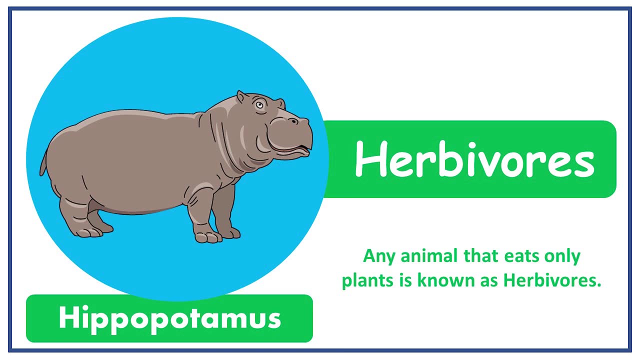 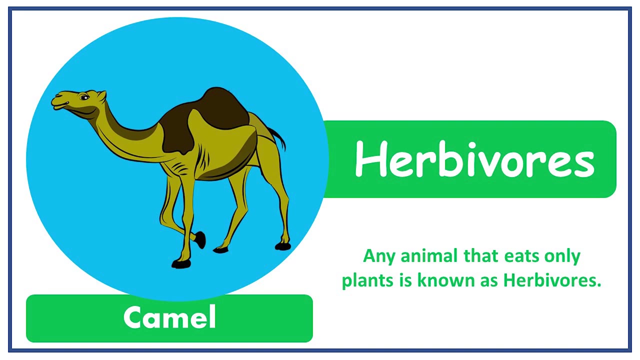 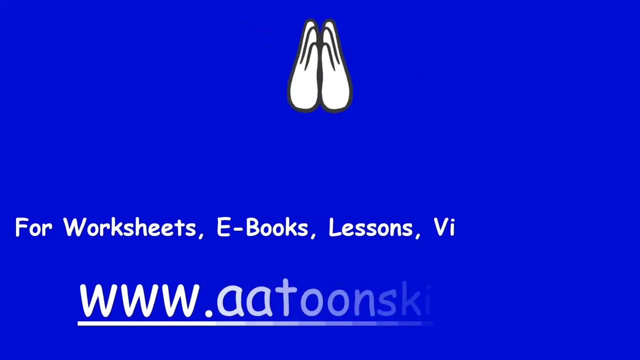 Ant is omnivorous, Crow is omnivorous, Cheetah is carnivorous, Hippopotamus is herbivorous, Camel is herbivorous. Subscribe the channel and press the bell icon. Click on the bell icon to receive notifications of new videos.